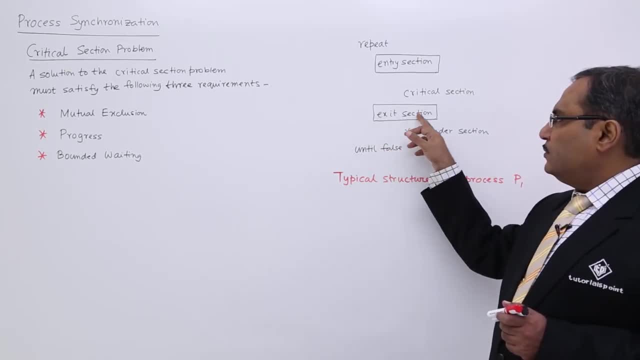 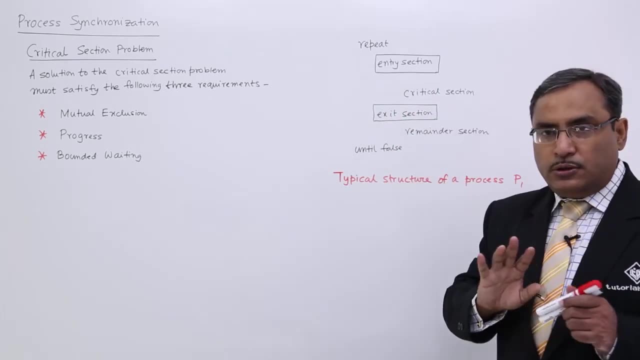 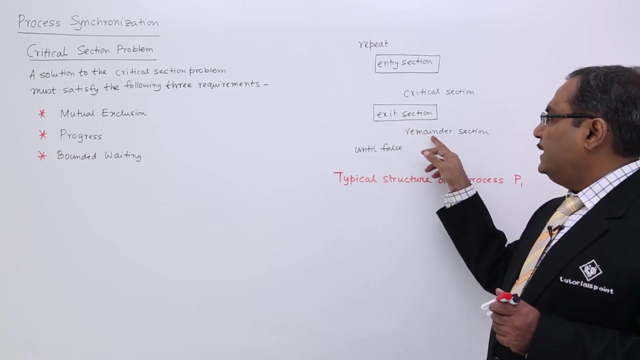 system that it is leaving the critical section and that is known as the exit section. So that is the main part. But after entering into the critical section, the process will not get terminated. It may have to enter into the same or other critical sections in its lifetime, and that is our remainder. 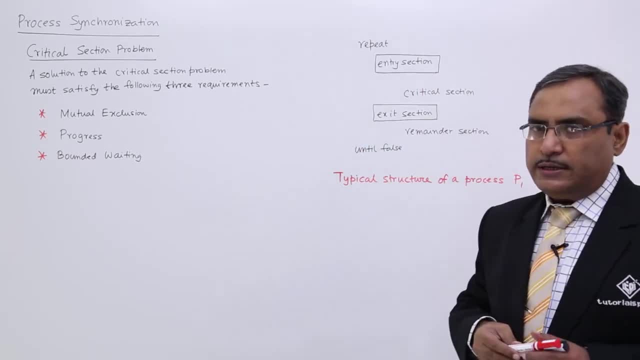 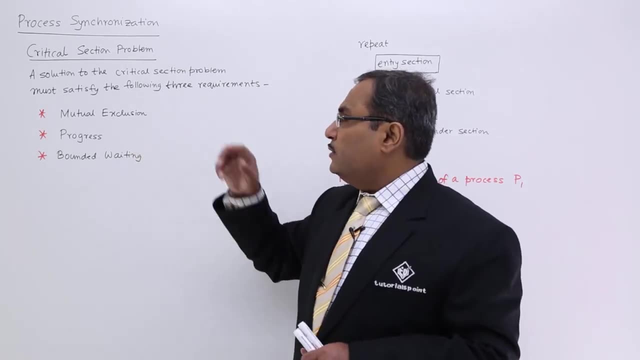 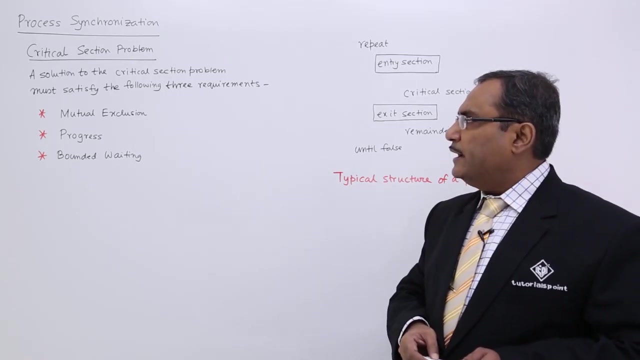 section. So in the remainder section again the process will try to enter into the same or differing critical sections. So that are the phases. are there Now? here we are going to discuss a critical section problem. A solution to the critical section problem must satisfy. 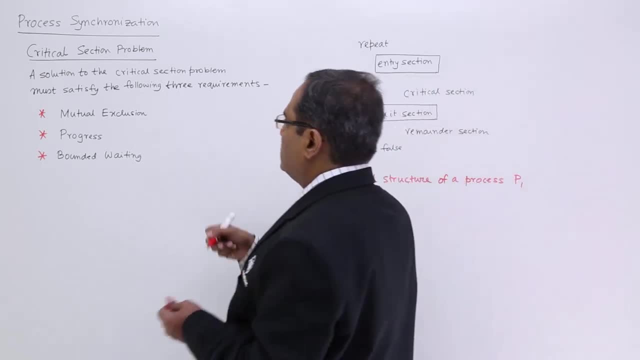 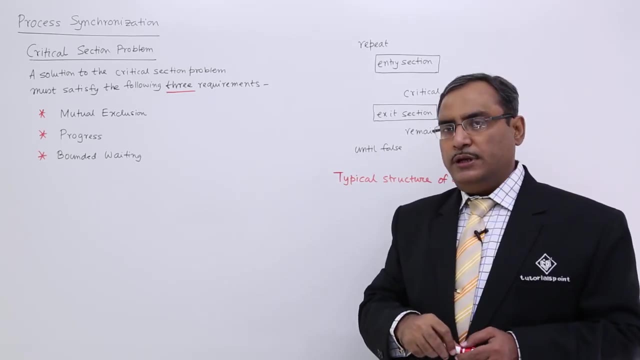 the following three criteria. First, it is a solution to the critical section problem. So there are three requirements. So the following three requirements are to be satisfied. So what are the requirements are there? one is known as a mutual exclusion. What is mutual? 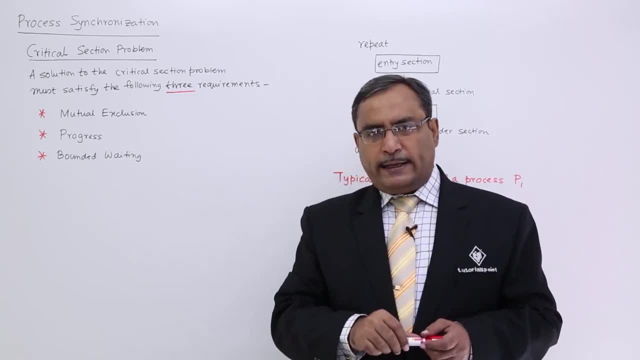 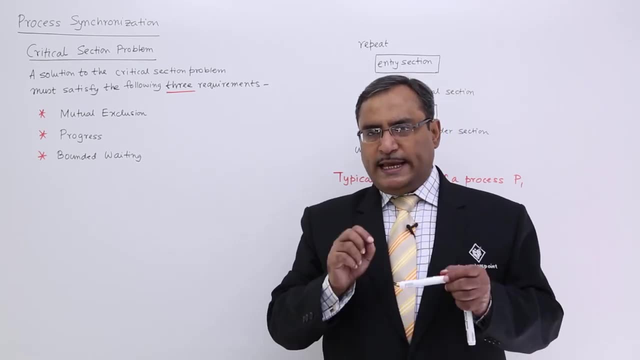 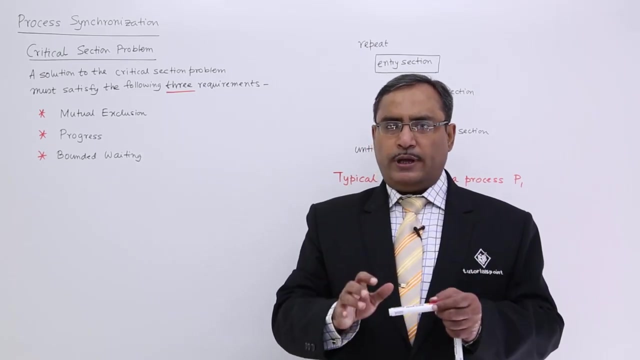 exclusion. Mutual exclusion means in the critical section at a time 1 and only one process can get an entry and that is known as the mutual exclusion. That means each and every critical section must be accessed by the process in a mutually exclusive way. That means at a. 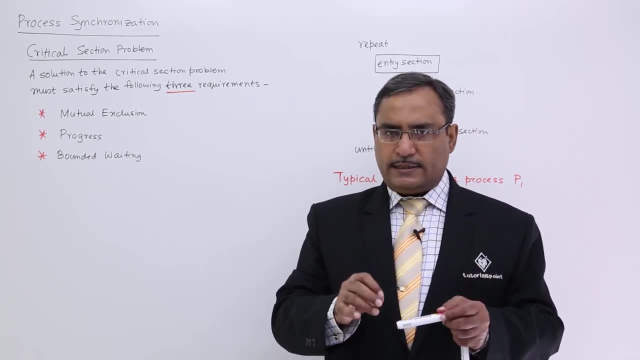 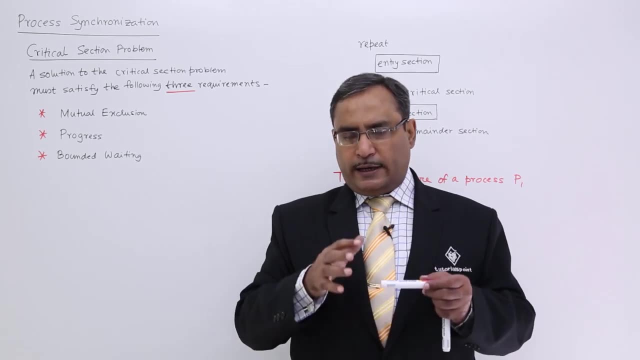 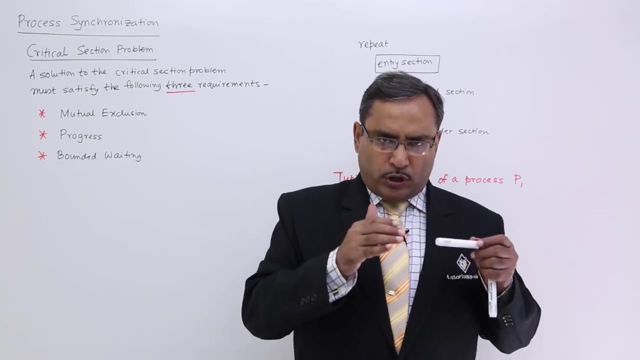 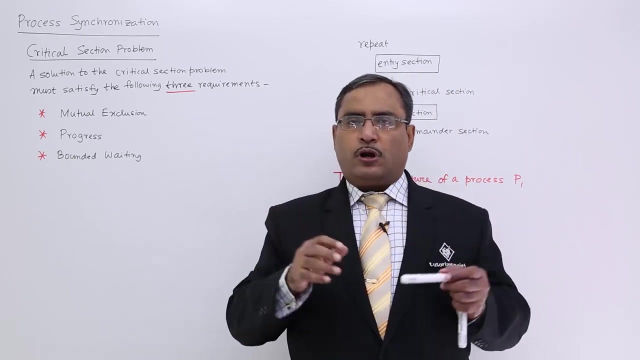 time only one process can enter, can access that critical section. next one is the progress. progress means, let us suppose a critical section is a critical section is vacant, that means there is no process is accessing the critical section and there are some processes are there waiting to enter into that critical section. then we should not wait for indefinite period. 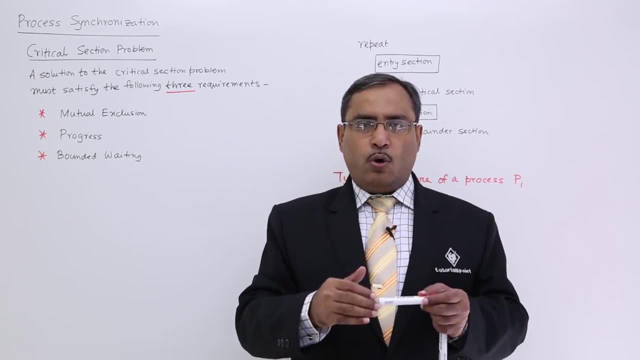 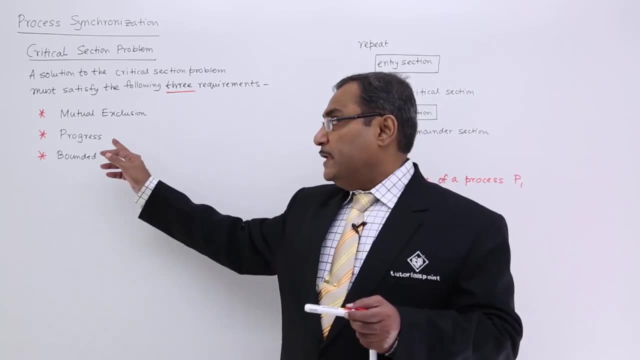 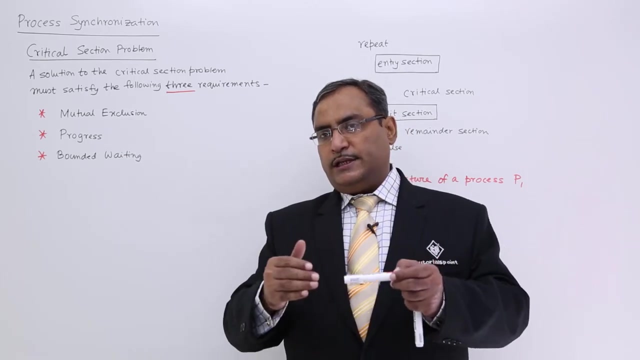 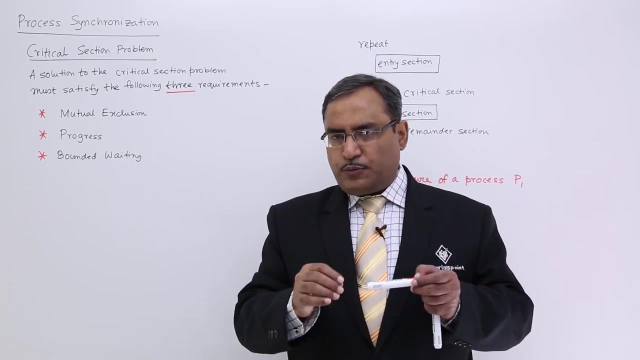 of time to do the selection that which process will go into the critical section. so that is known as the progress. so progress means the progress means a particular critical section is now free and some processes are existing to enter into the critical section. so the selection that which process will enter into the critical section, that selection process. 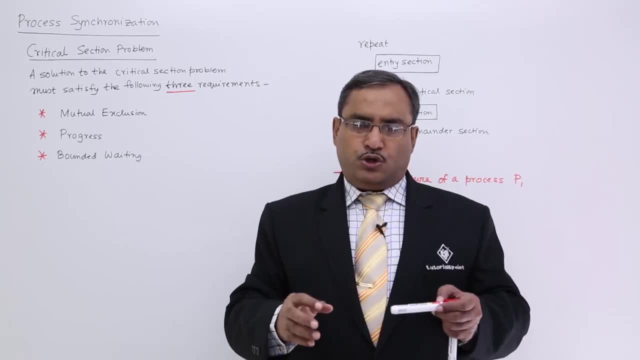 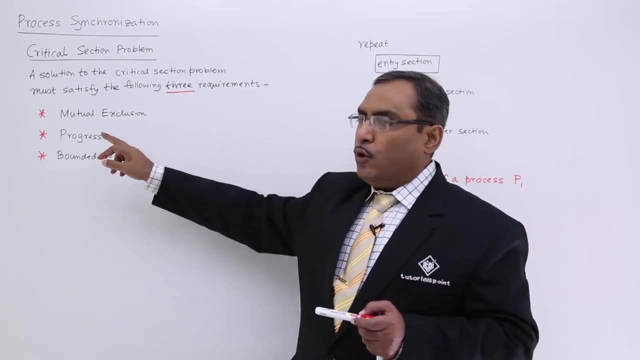 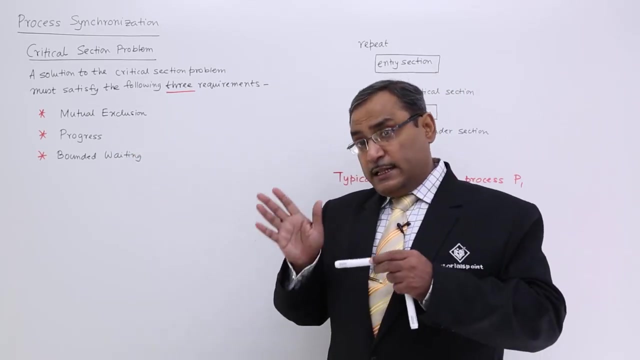 should not be postponed for indefinite period of time. it should be. the operating system should select which process should go into the critical section, and that is known as the progress. and also it is also true that that very processes which are in the remainder section- that means they had some critical sections earlier, they are now in the remainder section- should also 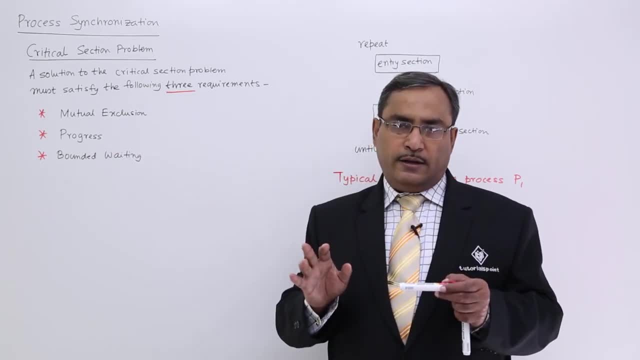 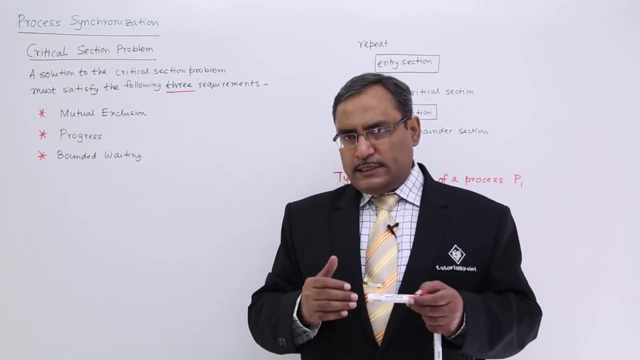 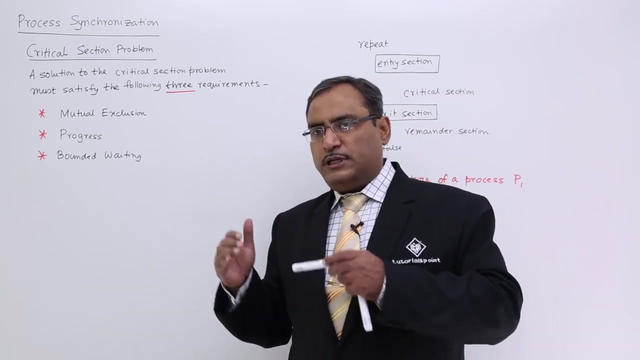 get a chance to enter into the critical section again, so that is also a part of the progress. in case of bounded waiting, what will happen? let us suppose a process has placed a request to enter into the critical section, but the operating system is allowing other processes to enter into the critical section. so there should be some upper bound up to which this. 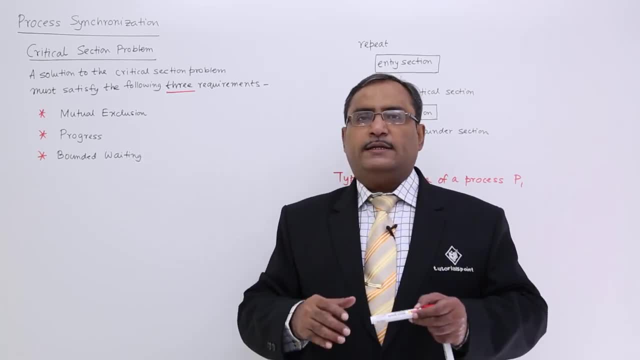 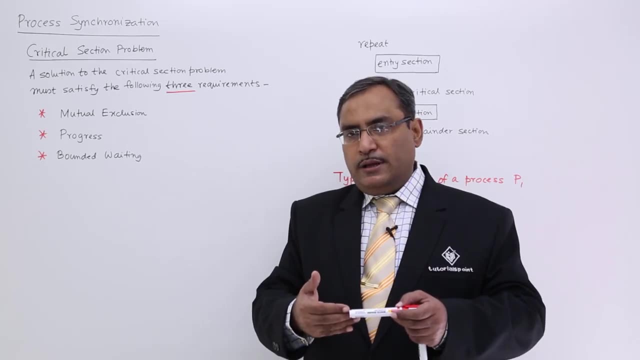 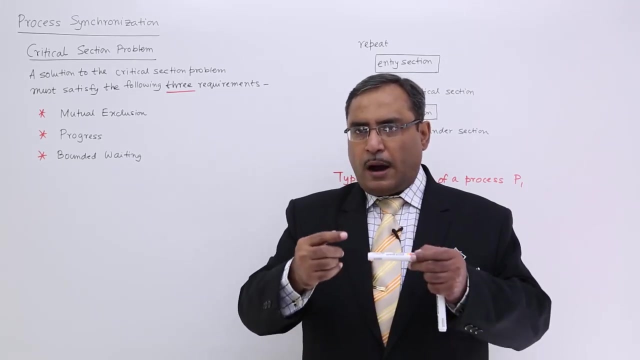 process request will be denied to get sanctioned. so that is known as the bounded waiting. that means i am requesting to enter into a critical section, but other processes are entering into the critical section. but for how many times i should get denied? there should have some upper limit and that is known as the bounded waiting. so in this way let me go for the conclusion. 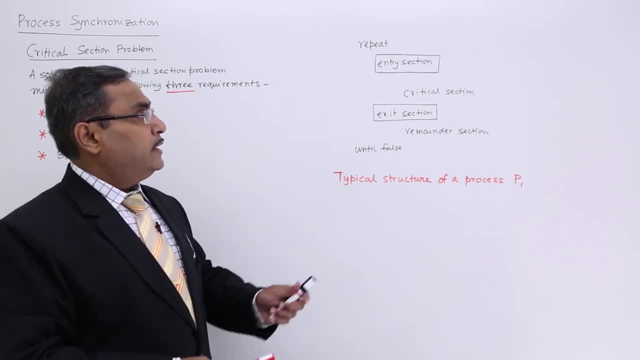 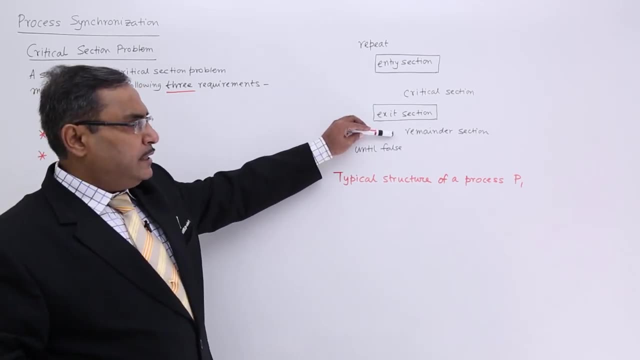 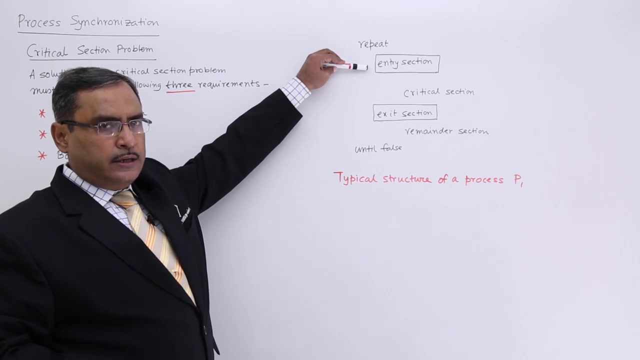 i am telling that in a process execution there are sections like entry section, then critical section, then exit section and there is a remainder section in this particular period of time again it will come into the entry section. that means it is requesting operating system to grant it to enter into the critical section, the critical section. 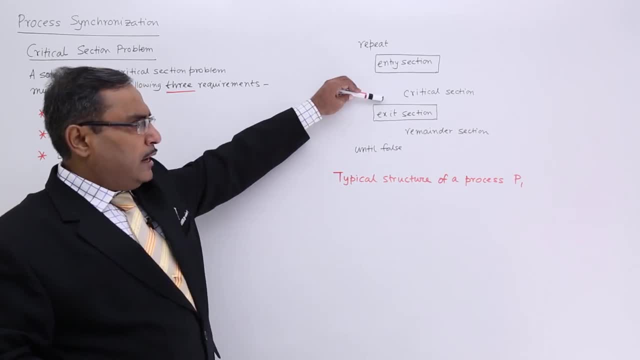 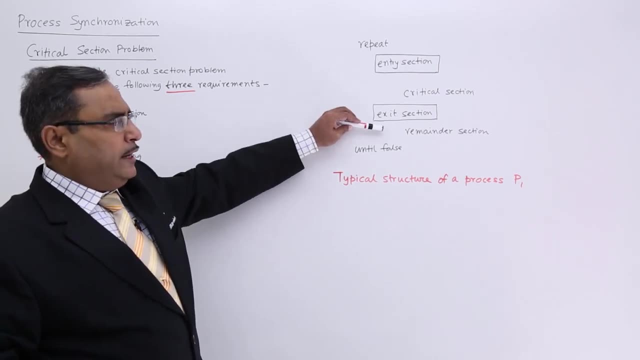 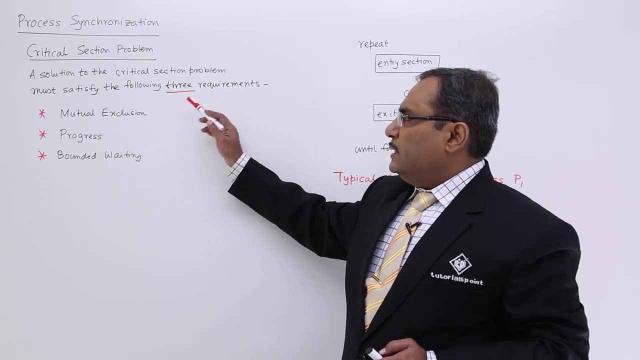 when it will be allowed, it will be using the shareable resource and while exiting from the critical section. then the resource will be released and operating system should be automated. it will find itself in the remainder section to enter into the same or other critical sections. the following three requirements are: each and every critical section must be: 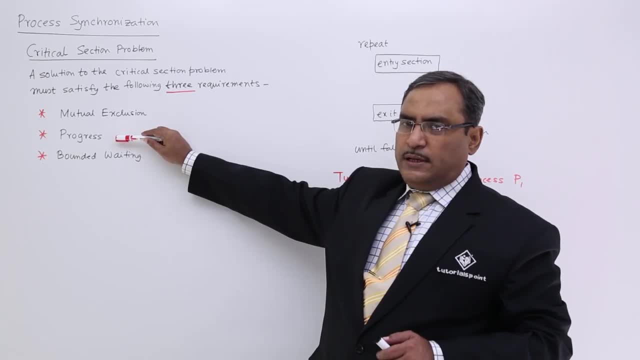 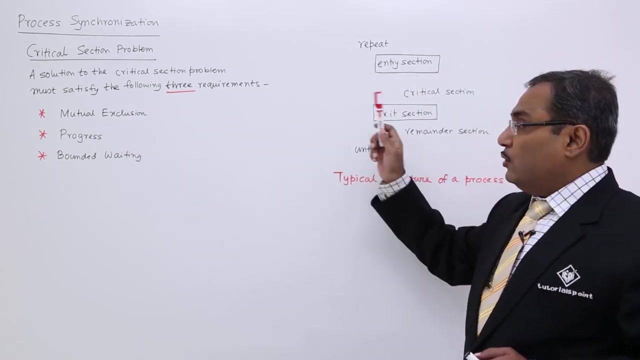 used in a mutually exclusive way. the progress means a critical section is free. processes are waiting to enter into the critical section, so the selection process should not get make them wait for indefinite period of time and those processes which are in the remainder section will also get a chance to enter. 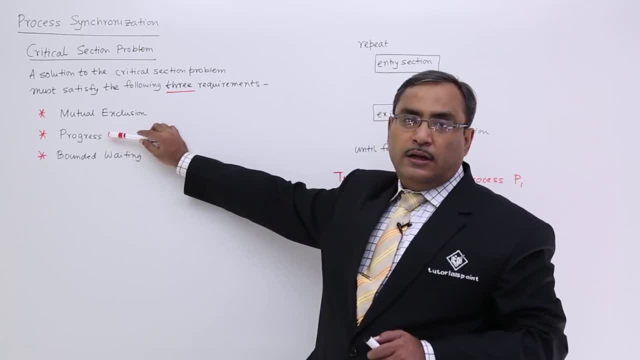 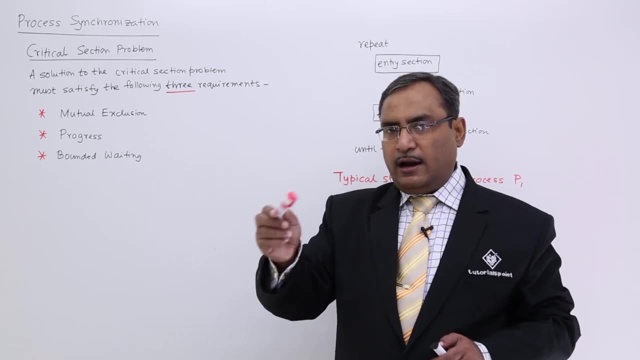 into the critical section and that they are falling under the point progress In the bounded waiting. a process has placed a request, but other processes are getting granted. So for how many number of times this process will get denied? that should have some upper bound. 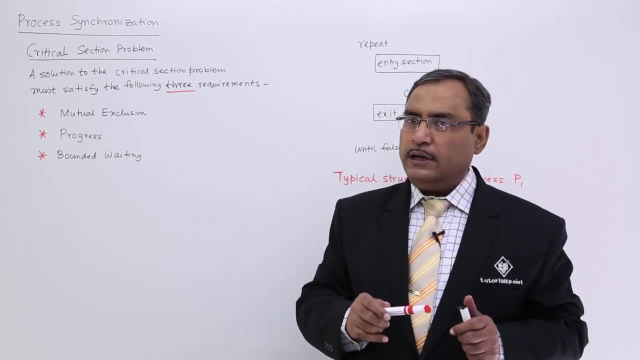 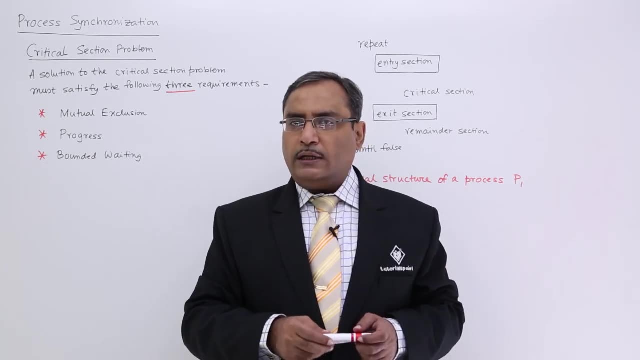 After that, this process must get an entry into the critical section, and that is known as the bounded waiting. I think you are getting this logic, what we have shared here, and we will be having other videos on this particular process, synchronization chapter. please watch them. Thanks for watching this video.